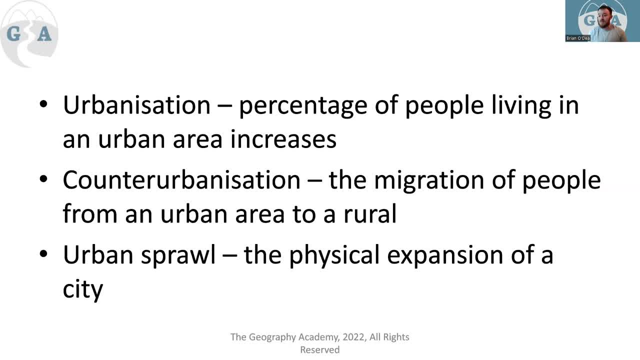 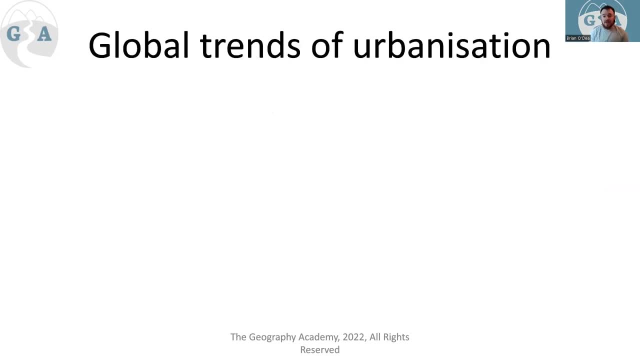 then we see people migrating back from urban areas to rural, to live outside of the city, So we see that as a trend, Mainly in developed countries. Urban sprawl, then, is just a term we use for the physical expansion of the city. We used it in the last video as well. So let's have a look at trends of urbanization. 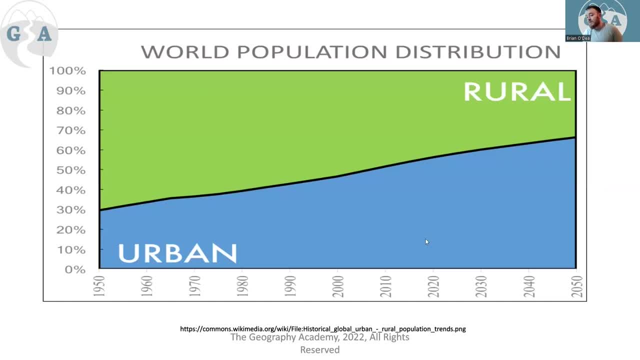 So we could see here that from 1950, all the way to what we anticipate in 2050 is a slow but consistent increase. Okay, Around 2020, we see that we've gone over the 50% mark, but this is. 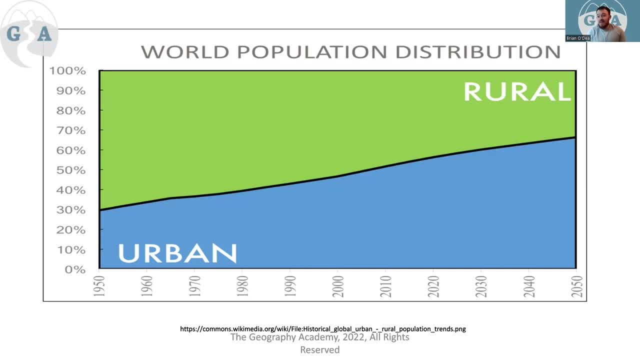 just a global average. we can see it shooting up from 1950s. Even in the 1950s most of the developed countries had a very high percentage of urban dwellers, like 70,, 80,, maybe more less developed countries, middle income countries suddenly getting very rapidly going through. 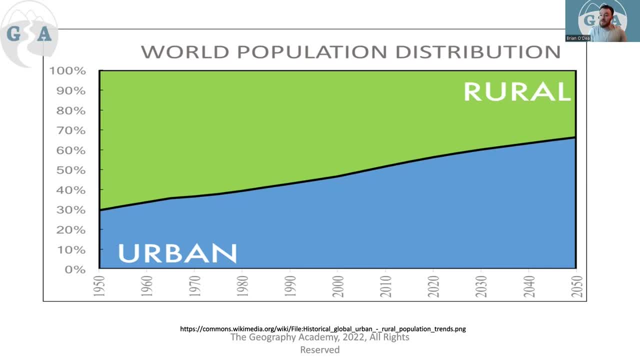 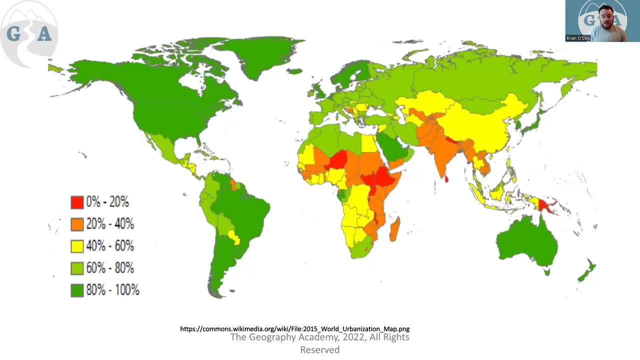 urbanization and having a higher percentage there. So their populations are quite large in a lot of cases And so they're increasing the world average then, So we can see where it's going, meaning it's a very critical thing to study right now If we're looking around at the general. 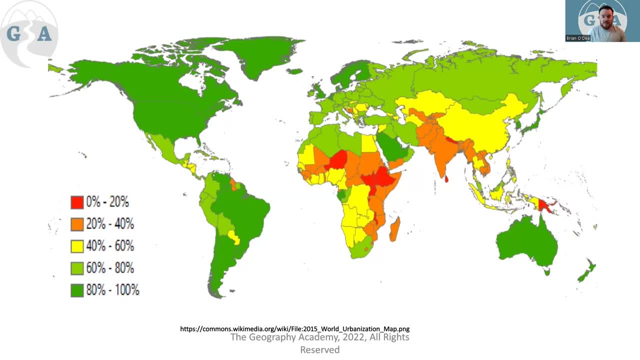 trends, then countries that are up in the 80 to 100% are often heavily industrialized countries or HIC, so Western Europe, Northern Europe and North America, a lot of South America as well, and certain countries then in places like South and Central Asia, but areas that are at its lowest. 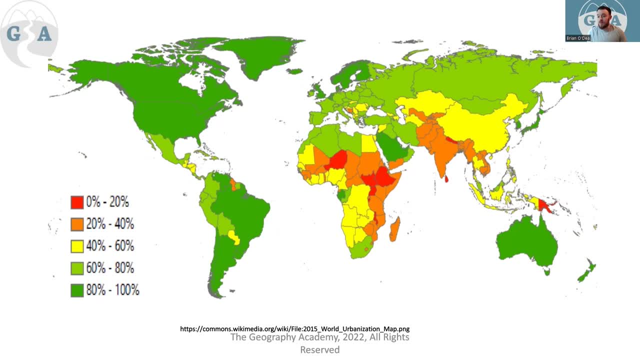 then we tend to have low income countries or even middle income countries or, to say, LEDCs often have a lot of people still working in the rural areas. Especially when we look at this region around South and Southeast Asia, we still see a lot of people. 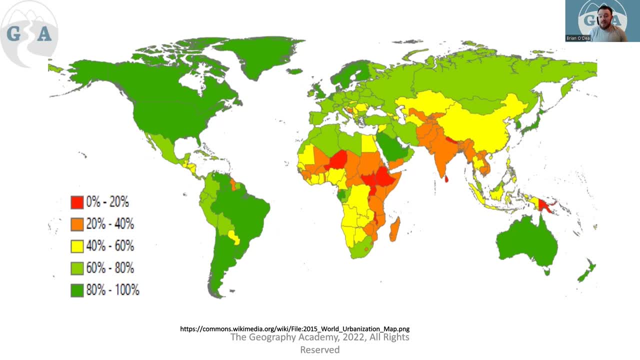 living in rural areas. They are meaning that a lot of people are probably still involved with the primary industry. Okay, so these changes have come about over a long period of time, but we can see the divide. So the countries in the yellow, then that are next in line to see a. 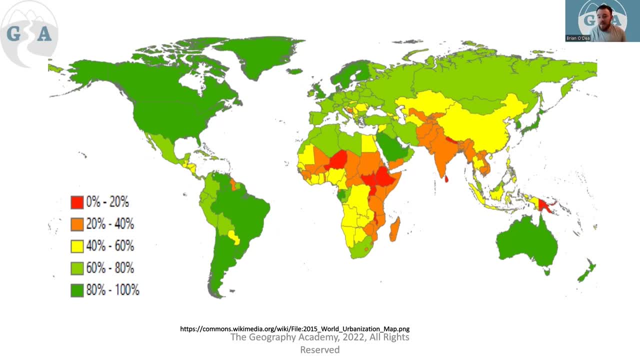 over 50% change in the population in the urban areas, And there's a few considerable countries that we have to look at, like China and Indonesia, for example, have very large populations, are just about to go through rapid urbanization, or going through it at the moment. 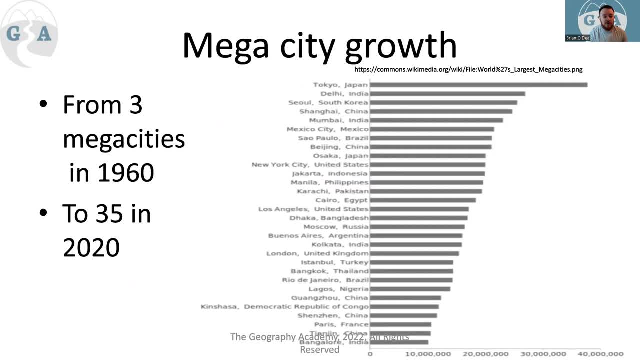 as well. we can mention that mega cities are growing, so a city with a population of over 10 million. we went from only having three of them in 1960 to having 35 in 2020. so have a look down through that list. you might be either very close to one or you might be actually living in one. 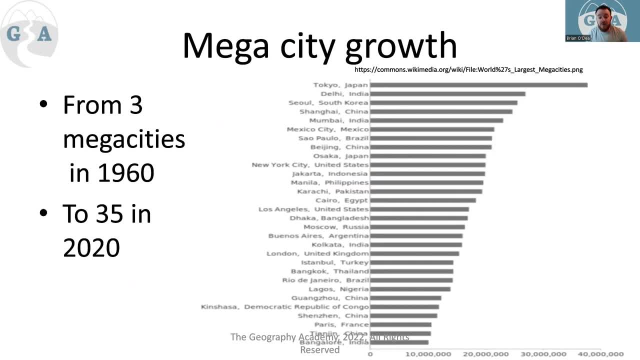 there's a good chance, as a lot of my students from all over the world come from one of these cities, so these cities, then, are known as mega cities with a population of 10 million. now, this just shows you that a very unique situation. when you have a population of that size, you've got a huge amount. 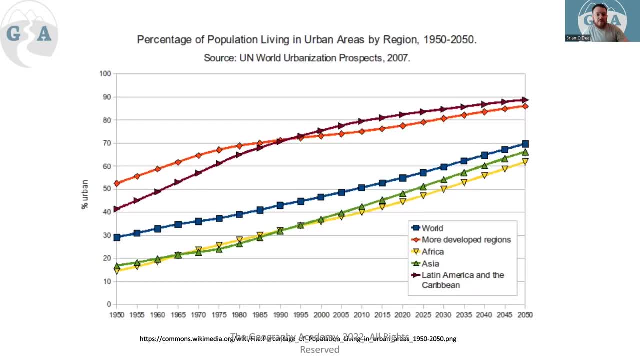 of issues that you have to deal with, so we're going to address some of those. we see the population in the world in regions. then if we look at the world on average, it's increasing. but, as i said before, if we look at the average of latin america, caribbean countries, that spiked very early. 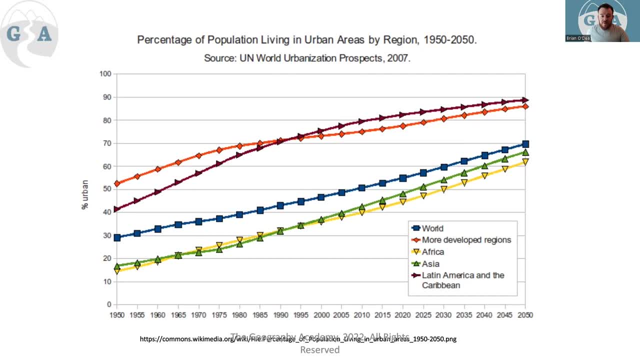 on after 1950, however, the more developed regions have always had a very high amount, both currently up there in an extremely high amount, uh, high, 80, high, 90 percent of the population. african countries, then, are the lowest, are they're intertwined in between asia and africa as the lowest there, but also a very rapid rate of growth as well. so even 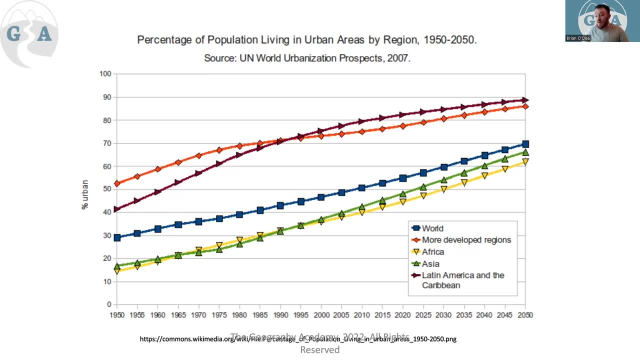 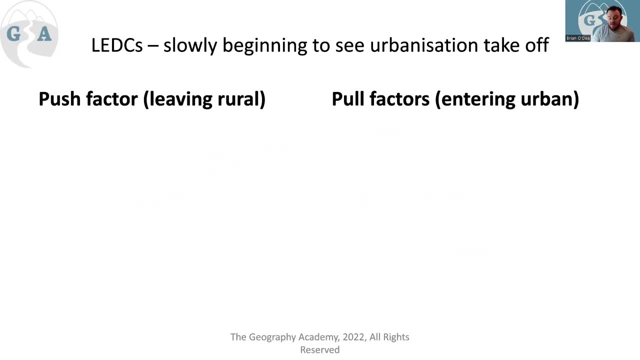 they'll see now they'll rise up and finally be a little higher percentage than we can see here. so the push factors and pull factors. so why do you want to leave the rural and come into the urban so reliant on subsistence? farming is not exactly the best thing in the world because you might have low. income, you might need to move somewhere else, and you might need to move somewhere else, and so that is another important factor that, as i said before, we've talked about. when you're trying to build a, the context, you're trying to find some foundations and you're trying to find some tools that could help you. 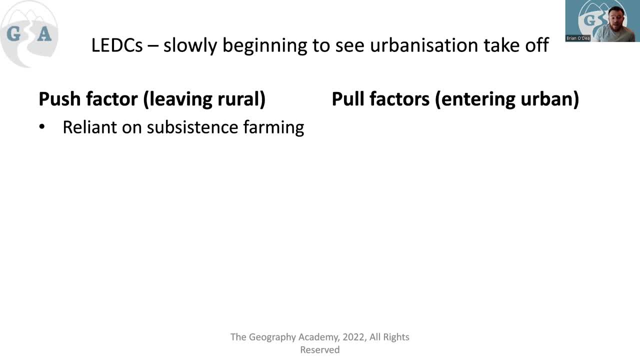 sudden change, drought, these types of things would mean that you're vulnerable to sudden changes. we also see mechanization of jobs in the rural area will change the industry slightly, meaning that less people will have jobs for you know manual labor, let's say communication through technology, wanting alternative lifestyles being exposed and understanding what life in the city is like, and